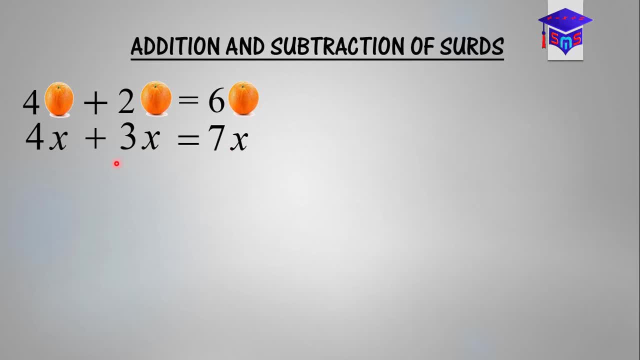 I'm going to get what? Seven eggs. What it means is that I have four eggs and I'm adding three eggs to the four eggs. So I'm having how many eggs? Seven eggs, Alright. Then again, if I have eight bananas and I take away five bananas, I'm going to have three bananas left. The same thing. 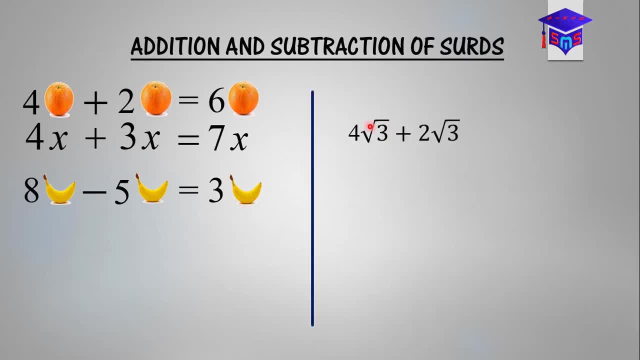 happens when you come to sets. If I have four root three plus two root three- because the root are the same- what it means is that I have four of the root threes and I'm having again two of the root threes, And so if I add two of the root threes to the four that I have, I'm going to get 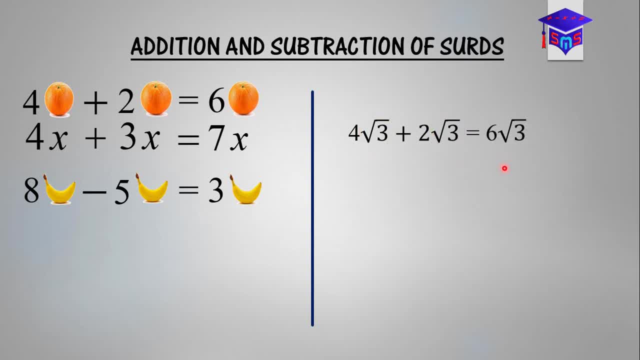 what Six, root three. What I just did was that I added the four and the what Two, And so four plus two give me six. then you bring what The root three. Alright, Then again, if you have eleven- root seven minus five- root seven, because the roots are the same, we can go ahead and subtract. 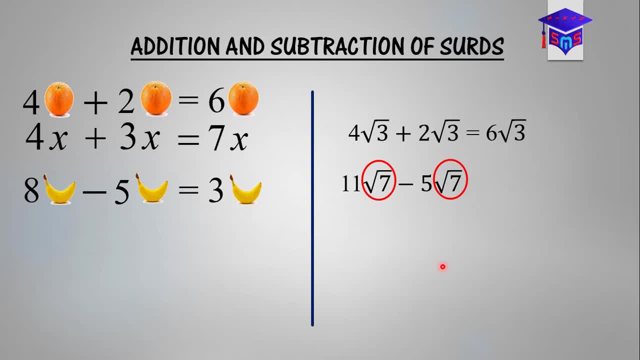 the five from what The eleven. So we are having: eleven minus five will give us six. then you bring the root seven. So eleven root seven minus five. root seven will give us six root seven. The only thing you do is that you subtract the coefficients, the second one from the first one. Alright, But 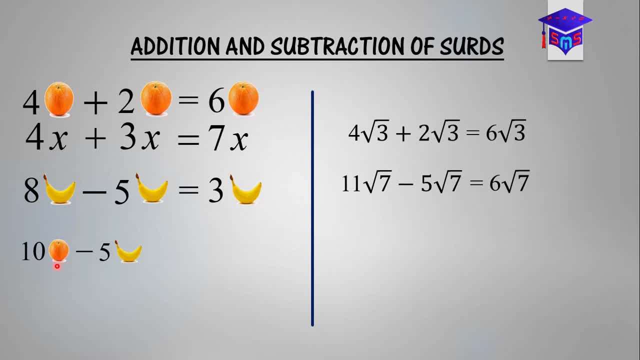 let's look at something. Assuming I have ten oranges, is it possible to take away the four bananas from ten oranges and get a single item? No, that's not possible. And also, if you have twenty-five oranges and you add five bananas, it's never possible to get a single item. But 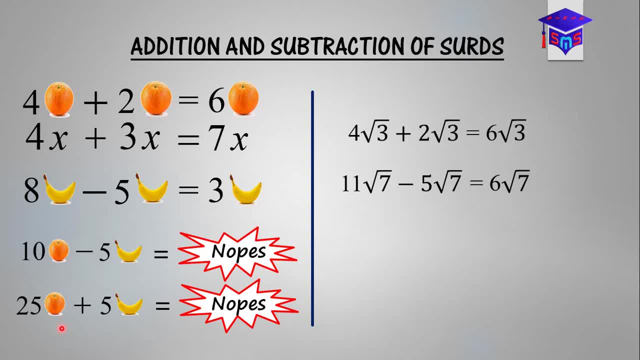 you agree with me that if I have twenty-five oranges in a box and I add five bananas, I'm going to have twenty-five oranges and five bananas? It can never add to give a single item like thirty oranges. No, there's nothing like oranges, bananas. And so the same way, in this case too, I'm going to have. 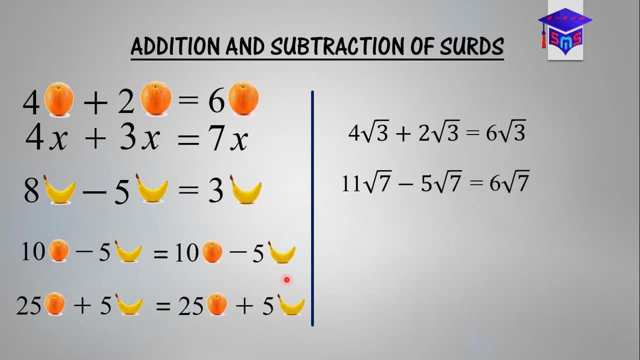 ten oranges minus five bananas. This can never add up to give me a single item. The same thing applies to, said: If you have five root six plus eight root two, because the roots are not the same, we cannot say we are going to add the coefficients or we are going to add the rational. 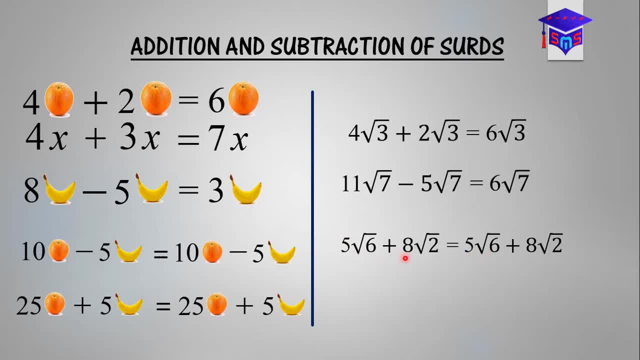 part, And so it remains the same. You cannot add them to get a single root, And so it remains the same. Same thing applies If you have seven root three minus four root five, because the roots are not the same, you can never subtract them. 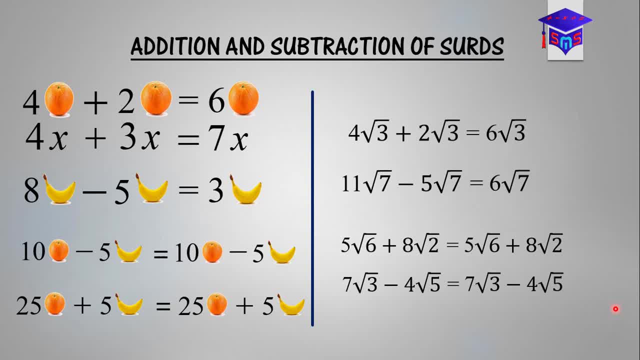 And so you're having the same thing. Seven root three minus four root five is equal to seven root three minus four root five, Don't even worry yourself. And so we can conclude that only like sets can be added or subtracted. Only like sets can be added or subtracted. 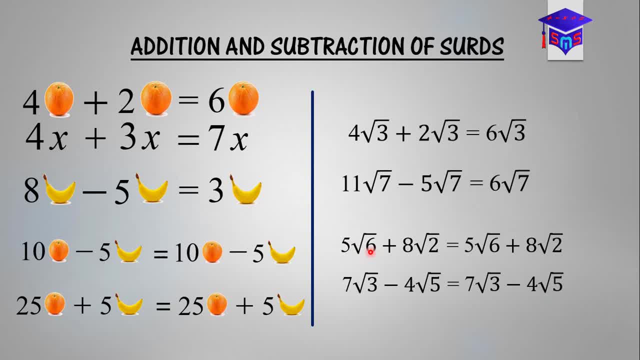 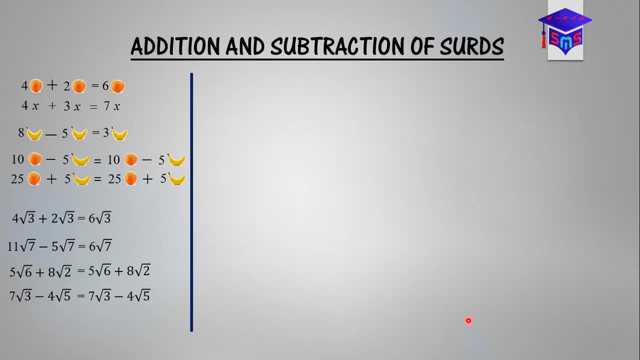 Only like sets can be added or subtracted, Unlike sets. like this can never be added to get a single unit. So in general we can say if you have m root k plus n root k, it's going to be m plus n root k. 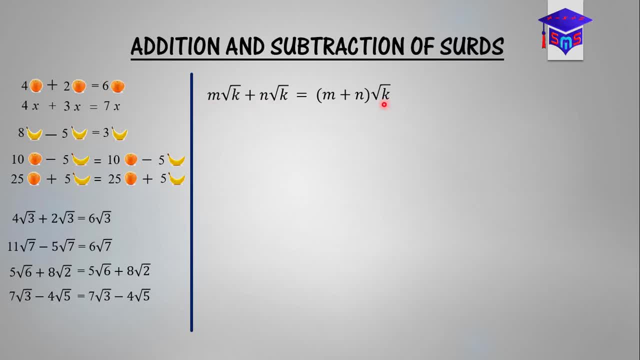 It's just going to add the coefficients. They maintain one of the roots. Likewise, if you have m root k minus n root k, you can guess what it's going to be. yes, you're right, you're going to have m minus n root k, and so these are the basic addition rules. 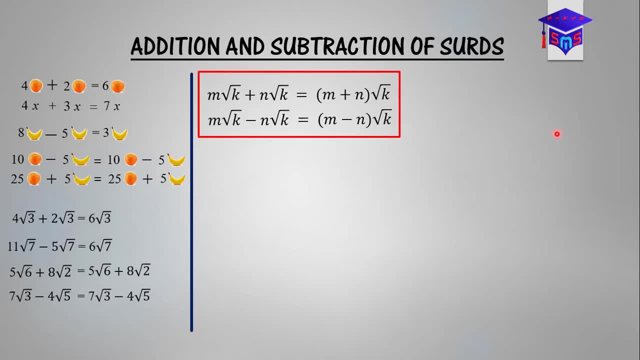 that will guide us to be able to perform addition and subtraction in sets. let's look at an example. if i have root 50 plus root 8, you agree with me that these sets are not in the simplest form, unlike these ones with their tweets. they are all in their simplest form. so then we have to reduce. 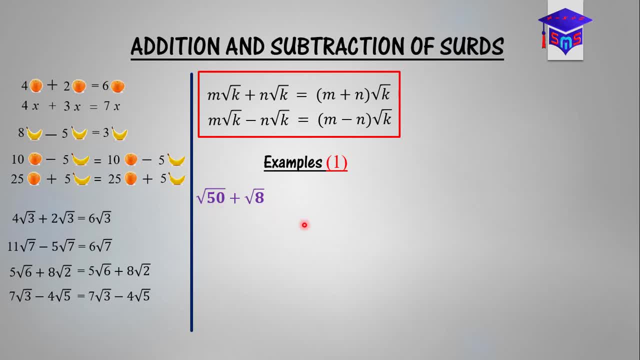 these sets to their simplest form before we go ahead and add them all right, so for the root 50, i'm going to have root 25 times 2, and then plus root 8 is root 4 times 2. good, then go ahead and each of them takes the root sign. the root 25 will take the root. this one also take the root this one. 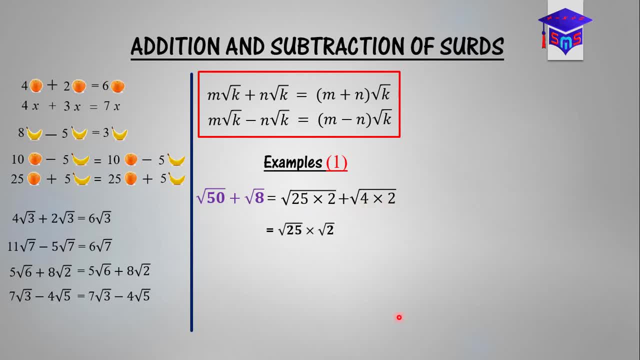 will take the root. this one also take the root. so we have root 25 times root 2, plus root 4 times root 2. if you are familiar with the system, there's no need to worry yourself about this step. then root 25 will give me what 5. then you bring the root 2, because it's already in the simplest. 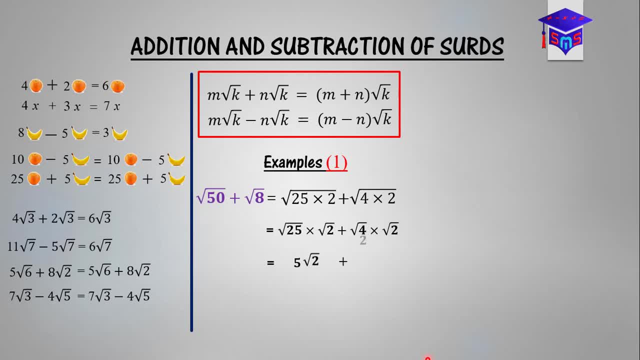 form. you cannot do anything to that. plus root 4 is equal to 2. then you bring the root 2. now both of them are in the simplest form, so we can go ahead and add them. and because the roots are the same means they are like sets, so we can add them and see. 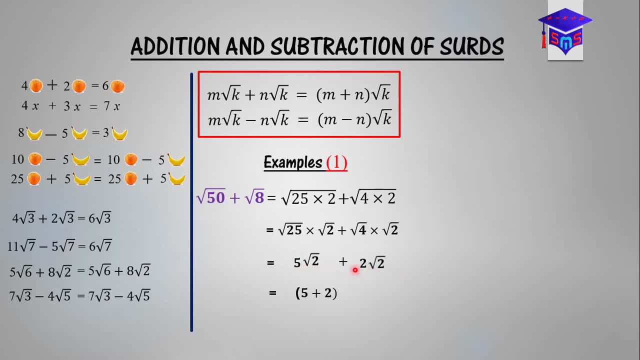 we are going to add 5 and 2, so 5 plus 2. then you bring the root 2, then 5 plus 2 is giving me what? 7? then you bring down the root 2. this is your answer. let's look at a second example. assuming 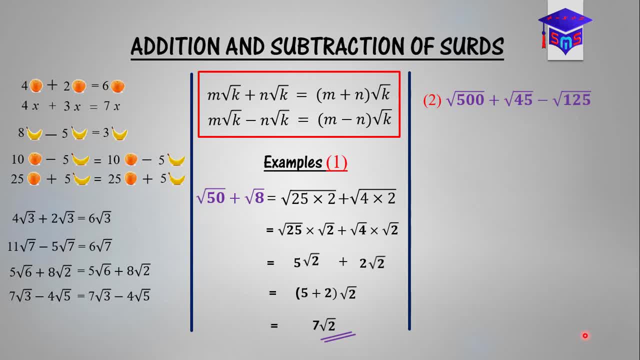 i have root 500 plus root 45 minus root 125. these roots, or these sets, are also not in the simplest form, so we have to reduce them to the simplest form before we go ahead and add them. add and subtract: root 500 can be written as root 100 times 5. 100 is a perfect square. 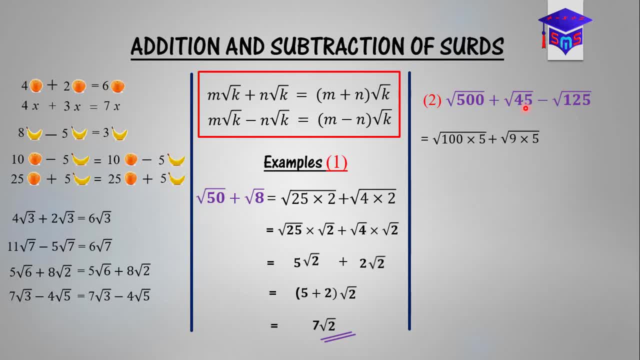 plus root 9 times 5, root 45 is the same as root 9 times 5. minus root 25 times what. 5 25 times 5 will give us 125. then we go ahead and each of them takes the square root sign. 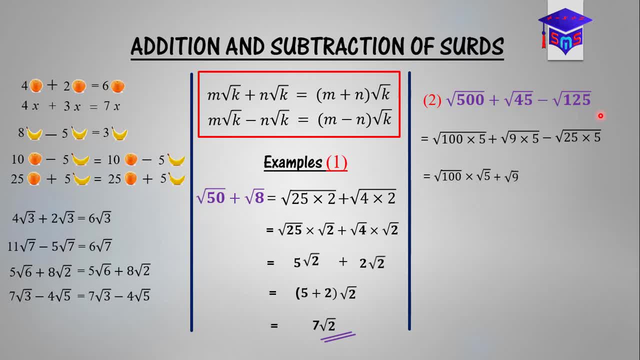 root: 100 times root: 5 plus root: 9 times root: 5 minus root: 25 times what: 5 times root? 5 times root, 5. you can skip this step. if you are familiar with how to go about it, it doesn't matter. you can. 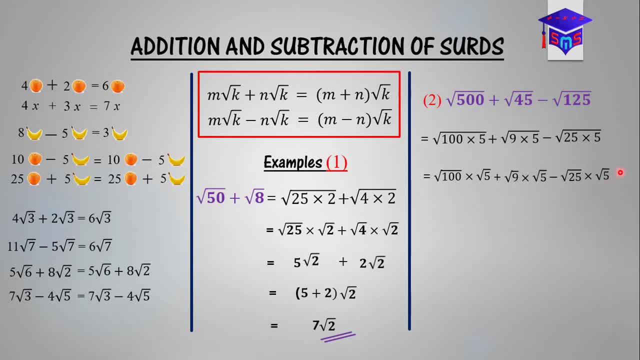 decide to skip this step. yes, root 100 will reduce to what 10. then bring down the square root 5, because root 5 is already in the simplified form. you can reduce it further. then root 9 will reduce to what three. root five. then root 25 will also reduce to what five. then you bring down root five. 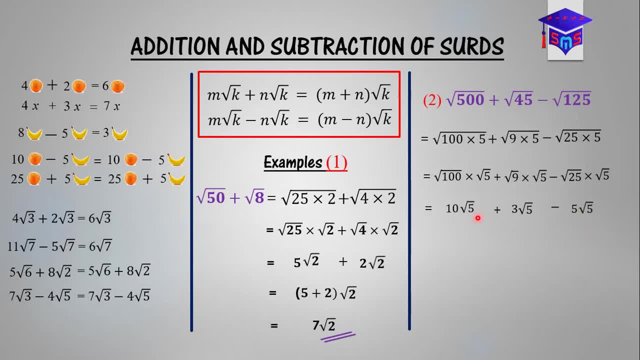 now this is in the simplest form, so we can go ahead and add and subtract the coefficient. now we are going to add the way to 10, then subtract 5.. all right, so you have 10 plus 3 minus 5. then you bring the root 5. okay, because they are like sets. 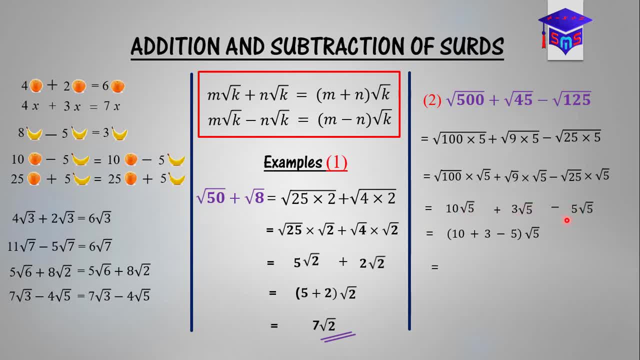 you can add and subtract their coefficients, all right, so this is going to give us 8, then you bring down a root 5.. that's your answer, isn't it simple? good, let's look at the last example. if i have 5 root 24 plus 11, root 7 minus 3 or 6, you see, if you look at this set, 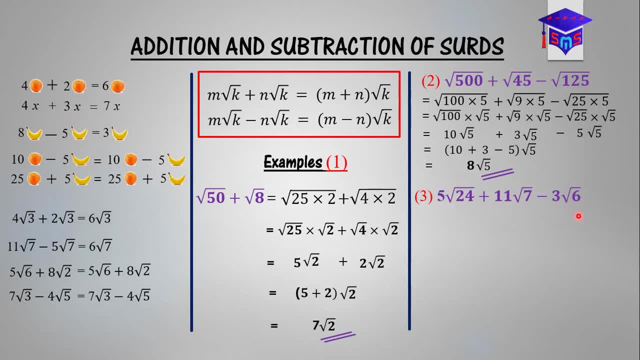 we check whether they are all in a simplest form. if not, then we have to reduce them to the simplest form before we proceed. when you look at root 24, it can be reduced further. i want to look at root 7. it's in the simplest form. you look at receive 2: it's in the simplest form, so we can't reduce. 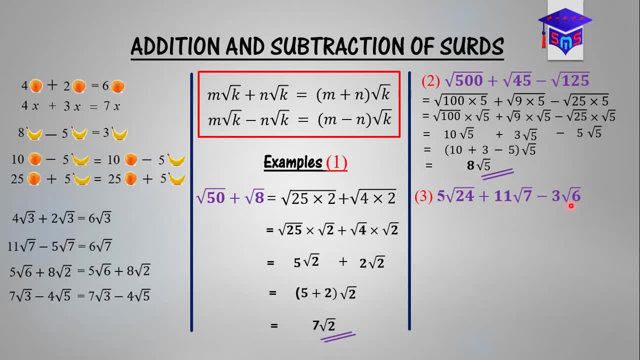 it further. so these two are already in your simplest form. these two are already in your simplest form, But when we look at root 24, we have to reduce it further. Okay, so can we write this first term in this form: Five root four times six. 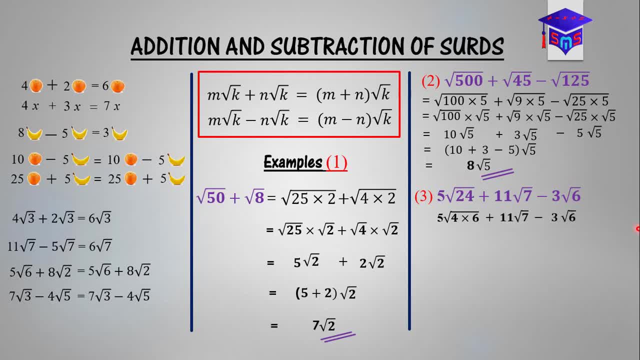 Four, six is what 24.. Then we bring down the other ones, because they are already in their simplest form. All right, let's simplify this further. You can go ahead and write this in this form, then bring down the other ones. 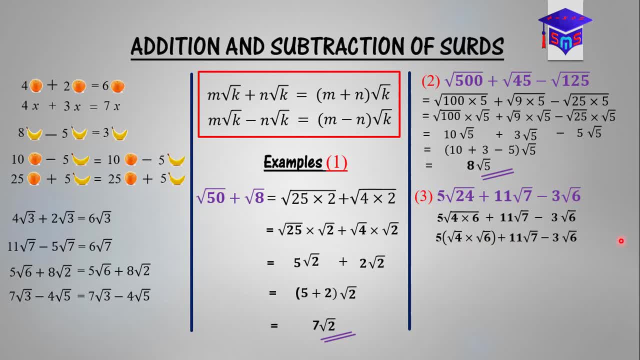 You can start to skip this step if you are familiar with how to do these things. Then again we can write root four. we reduce to what two. Root four is the same as two. okay, You bring the other terms. Then the two will multiply the five. 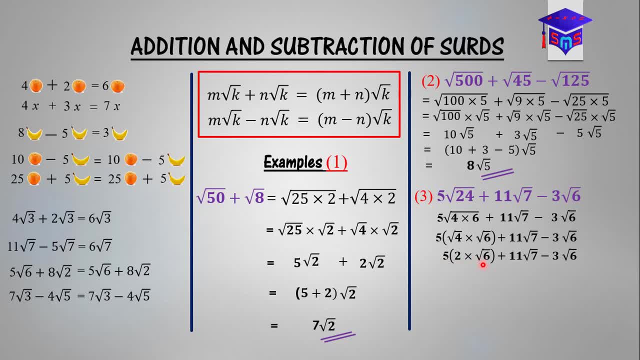 The two, multiply the five, of course. So you have five times two root six. So five times two will give us what 10.. So you have 10 root six and you bring the other terms Now you see that we have 10 root six plus 11. 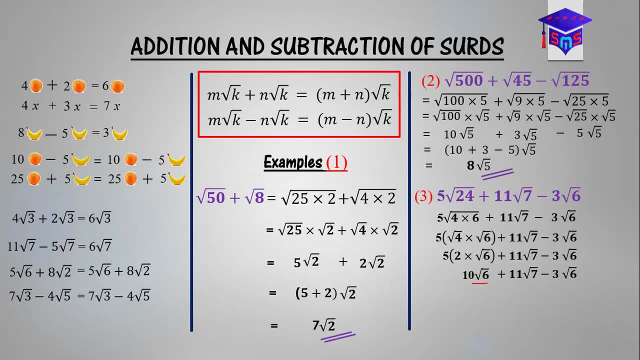 root seven minus three root six. These two are like sets, You see that Good. So we can go ahead and rearrange this to have 10 root six minus three root six plus 11 root seven. So we can go ahead and then subtract these two. 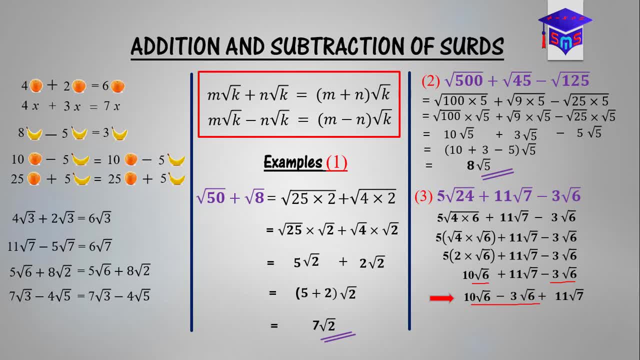 You can subtract three root six from what 10 root six, because they are like sets, because the roots are what the same. so we can subtract them, All right, and we are getting 10 minus three root six, plus what 11 root seven. 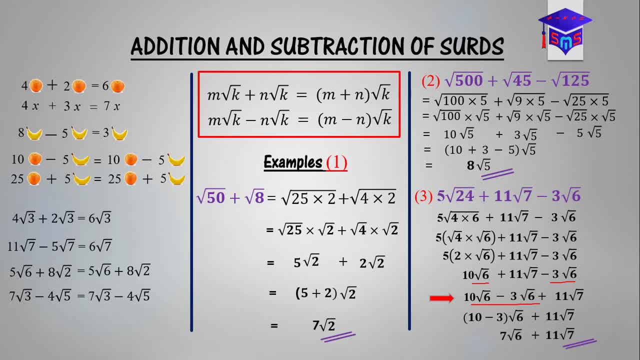 Then this one: we reduce to what seven root six plus what 11 root seven. That's your answer. We cannot add this to that. We cannot add 11 root seven to seven root six, because they are not like sets, And so this is your answer. 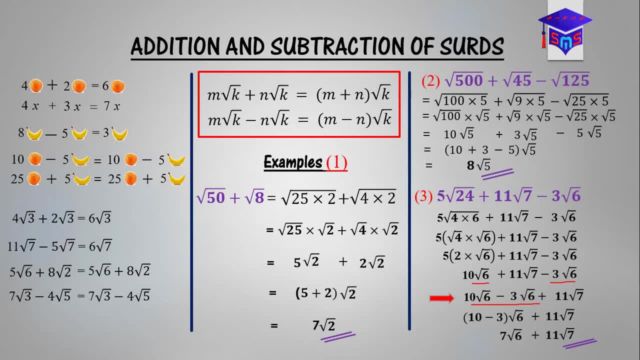 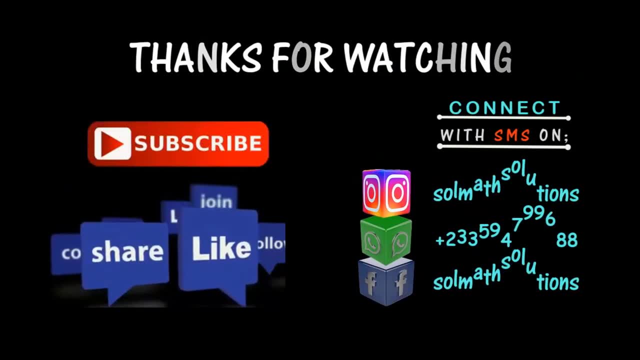 All right, thanks for watching and I'll see you in the next section where we talk about multiplication and division of sets. So stay tuned and I'll see you in the next lesson. Bye-bye. 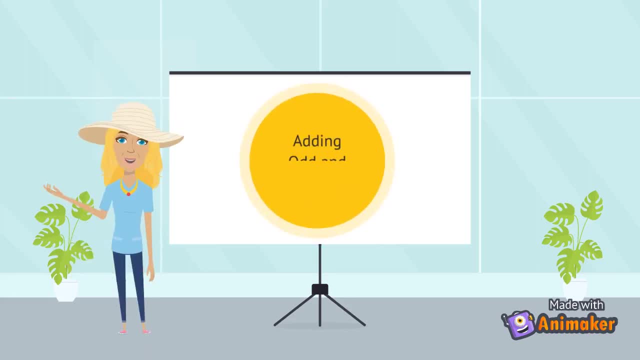 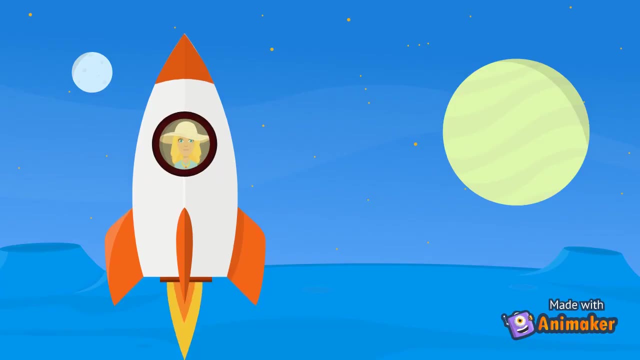 Hi, it's me again, Mrs Romaya, and today I'm going to talk to you about adding odd and even numbers and what the rules are. Let's put it this way: it's not rocket science, which means it's pretty straightforward. 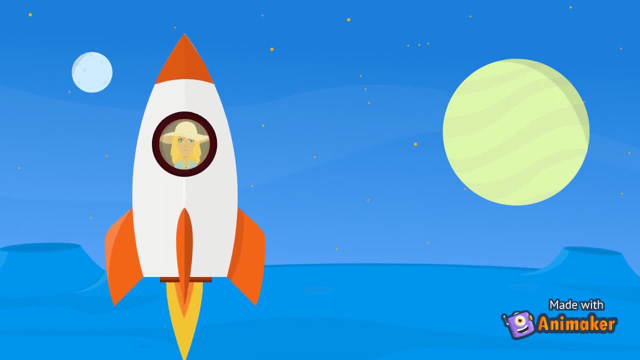 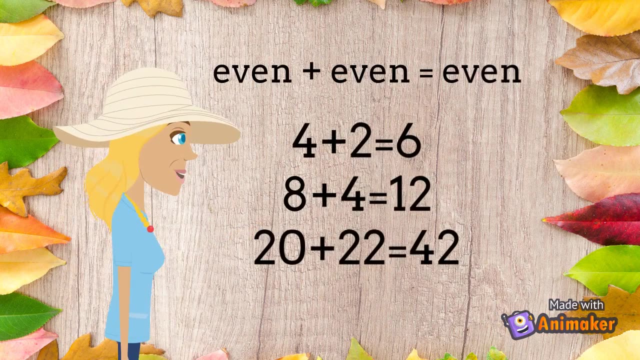 There's just a few simple rules and I'm just going to show them to you. It's very easy: When we add an even number to another even number, we get an even number: 4 plus 2 is 6,, 8 plus 4 is 12, and 20 plus 22 is 42.. 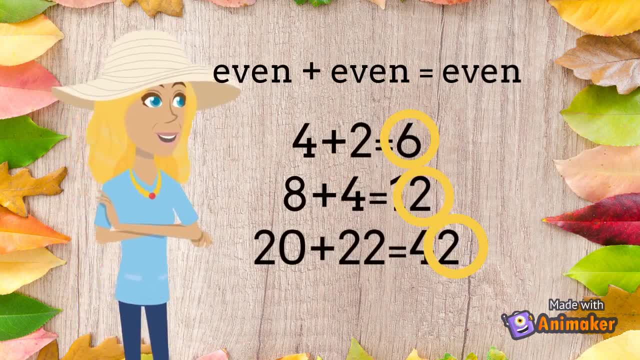 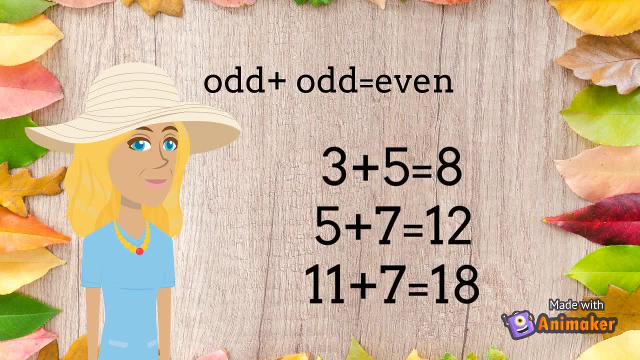 We know they're even numbers because they end in 2,, 4,, 6,, 8, and 0.. Look at these. they end in 6,, 2, and 2, so they're even numbers. So when we add two odd numbers, what happens? We get an even number. 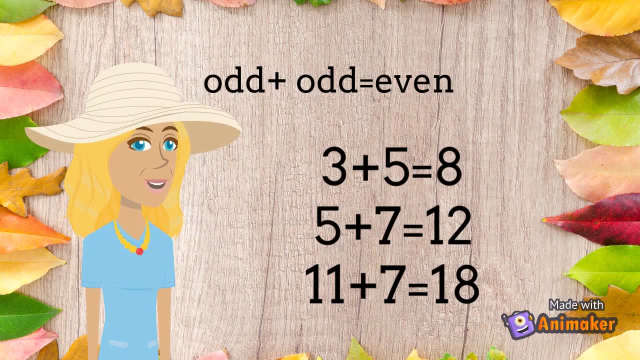 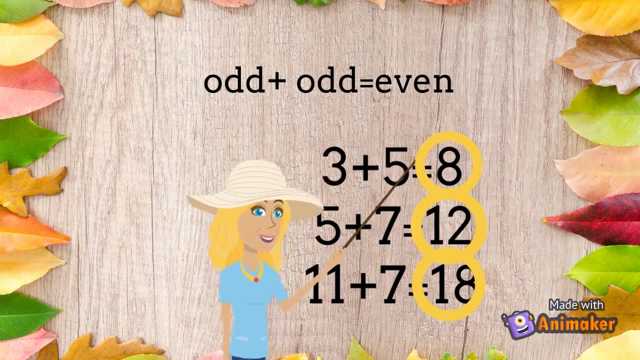 Look at these examples. We're getting even numbers when we're adding two odd numbers. Okay, so here we have 3 plus 5, which is 8, even. 5 plus 7, which is 12, even. 11 plus 7,, which is 18, even.